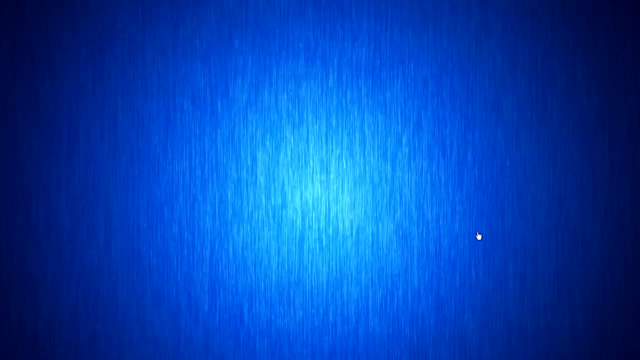 they work and just a little bit of understanding can make tuning decisions on your quad much, much easier to make For our flight performance. really, the two most important terms are P and D. P term is kind of the main important driving term. So if we say, have our stick centered, we're looking at zero degrees. 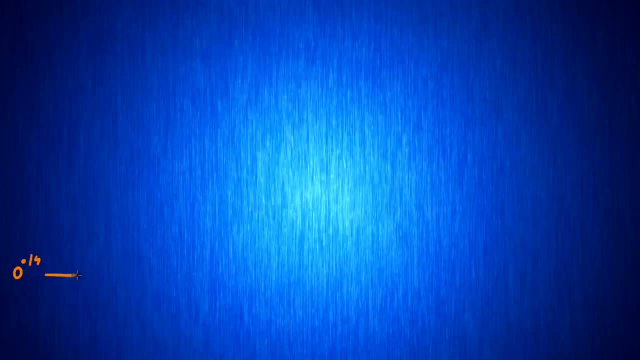 a second and we want to do a snap roll. So we very quickly ramp up to 600 degrees a second and then hold the stick there. If we look at what just the P term will do and say, our red line here is what P term gives us. the P term looks at how 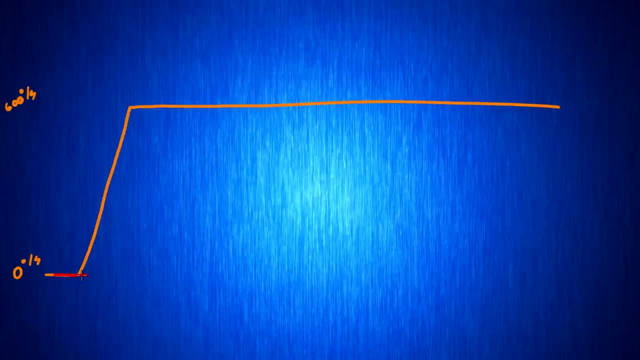 far away we are from the destination. Here the P term sees the destination is getting further away and it's going to start accelerating towards it. And as we come here, the destination is really far away. So the P term is going to say like, hey, we need to get moving this direction. We're really far away And it's 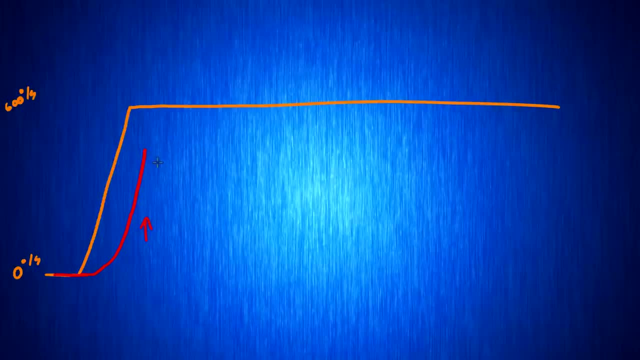 going to keep going. And here we're getting closer. So the P term is going to say, hey, we're only a little far away, We don't need to accelerate quite as much, So it's going to accelerate less. And then, when we're right up here, it's going to say, hey, we're pretty close, We. 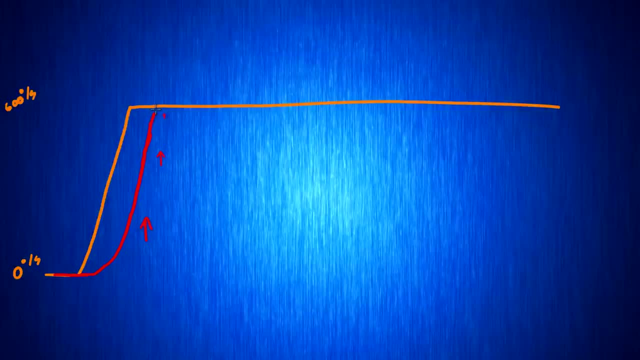 only need to move a tiny tiny amount over there, But because we're moving a physical thing, we have momentum and it's going to keep moving, even though the P term is not trying to accelerate us anymore. We have all of this motion that we've built up from earlier. 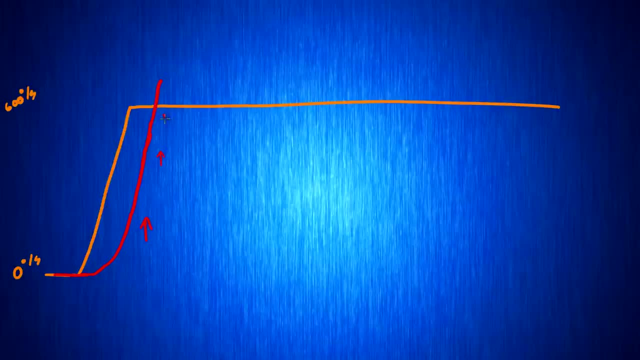 And so we're going to actually blow right past the destination because P term doesn't know to slam the brakes And try and slow us down the other way, And it's going to sit here and say, hey, we need to go this way. We're past the destination again, But the P term of course doesn't. 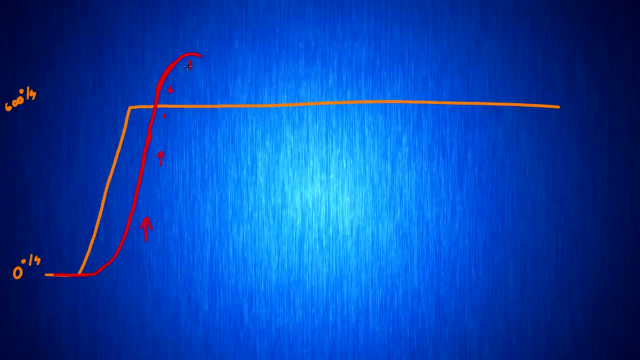 work instantly And so it's going to take some time And we're going to cancel all of our momentum out. And then it's going to say, hey, we need to go that way again, And so on and so forth, And it's going to give you this oscillating thing when you hear P term. 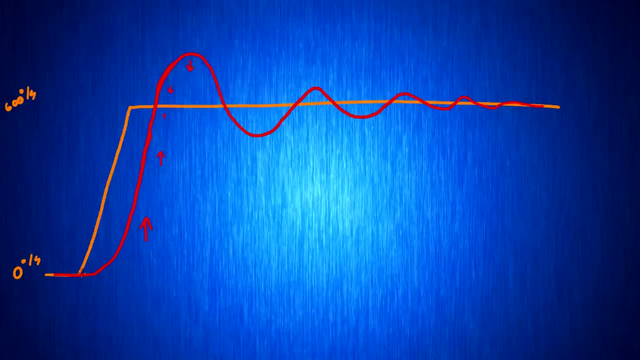 Oscillations. This is the sort of effect that you get. It takes time to hit our final destination, But P term doesn't know to slow down And so it overshoots and compensates by trying to go the opposite direction And it does not settle on. So you see, we've been. 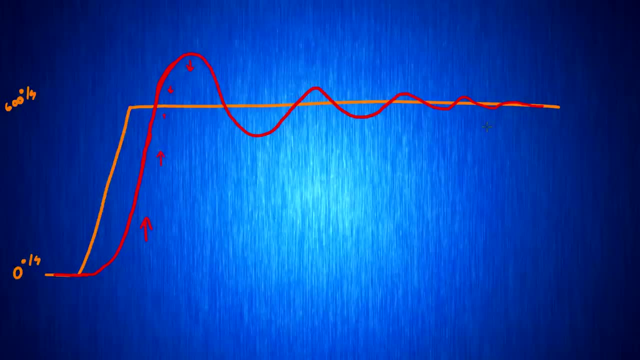 holding the stick for a long time and the quad is just bouncing back and forth, And this happens very, very quickly. If your P gains are really, really high, you may have a lot of oscillation. If your P term is too low, it'll see that it's trying to do, But if your term is very 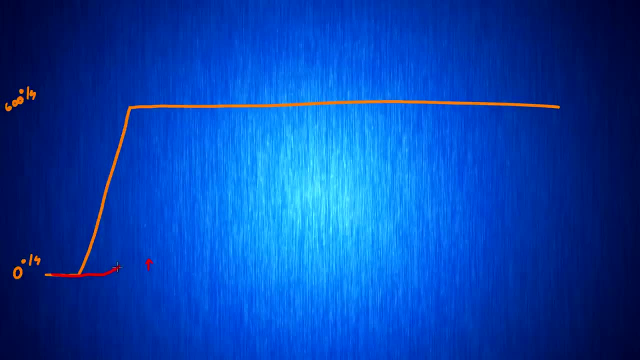 low, then you're only allowing it to say: we need to move a little bit in this direction. And so it's only going to push a tiny tiny amount all through here And we'll slow down because we are losing our momentum And as we get closer, the P term is also getting. 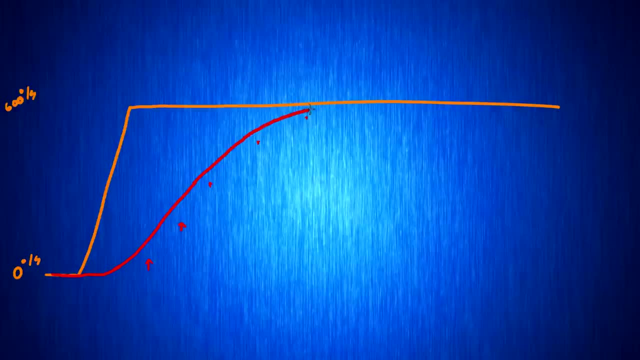 smaller, And so you can see what we end up getting is we don't necessarily overshoot, But it takes us forever to hit our target And this leads to very sloppy control and loss of stabilization. Things interfere with the quad. It can't move quick enough to react. 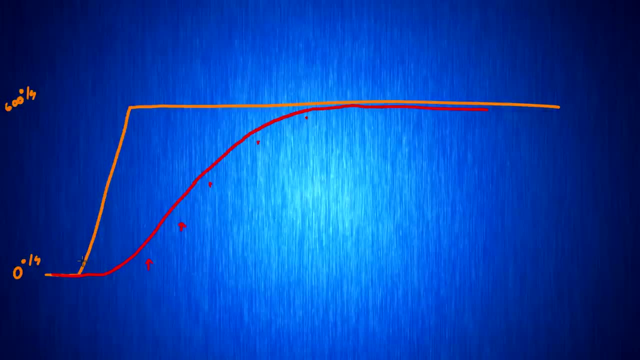 So that's the problem with P term: If you have too little of it, you have very poor control and it doesn't react very quickly. And if you have too much of it, you get nice and sharp control but you get massive overshoots. 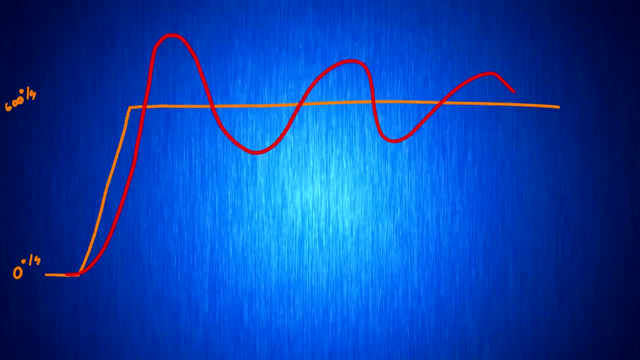 The D term helps us compensate for this. What the D term does is it kind of looks at how quickly we are approaching our target. So when we're down here, the P term is cranking it up and saying we need to go up here and say we're at this point. the P term is saying 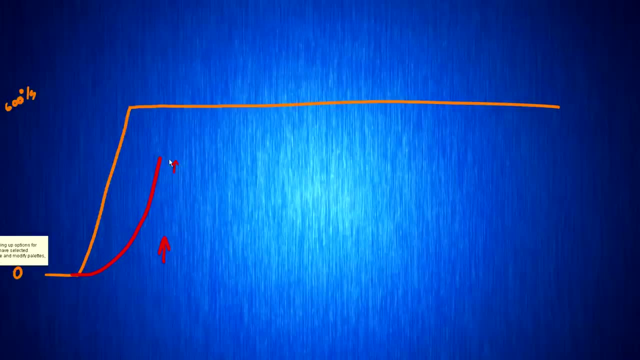 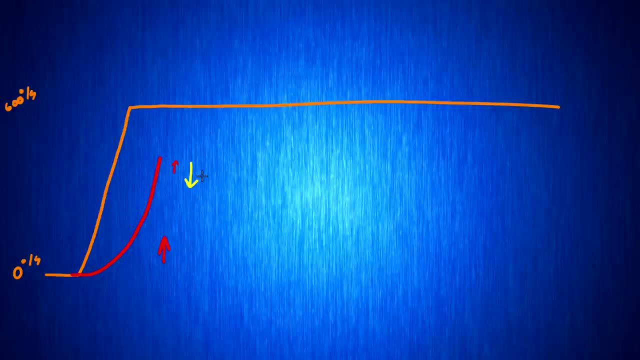 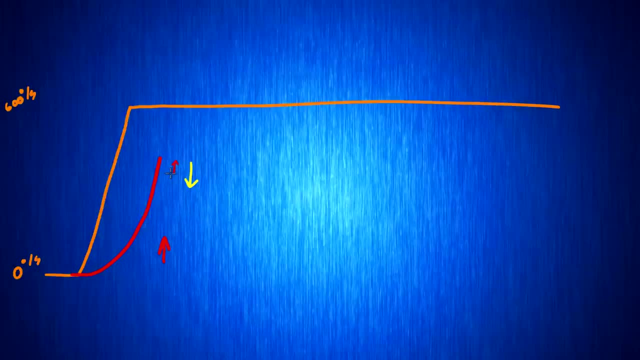 P and the D get added together, That becomes the. you add all the terms together, That becomes the pit sum that actually drives the motors. But so we'd say we have a little bit of a P term here. as we're getting closer We're. 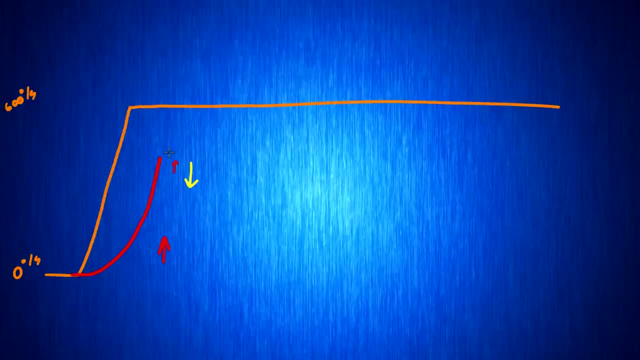 not too far away. So the P term uh says: and we only to accelerate a little bit cause we're not too far Um. the D term sees: Hey, we're approaching very quickly, We need to start slowing down. And what this gives us a final number. If you add, say, a small number and a big. 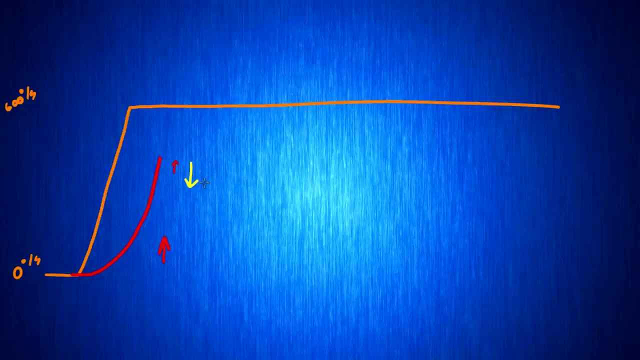 number we or a- um, you know, a small positive and a big negative. you see, it's going to give us a mostly negative number, So it's actually going to start slowing. uh, the the motors down. 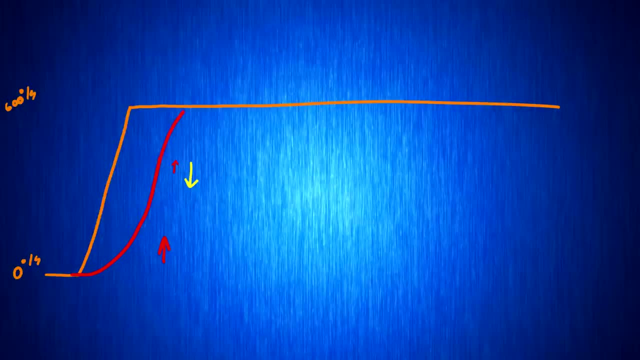 So we don't try and overshoot, So we start slowing down and the D term says: okay, we're approaching a little slower, We need less reverse force. And the P term is still blindly doing its thing And it said: well, we're pretty close, So we only need a tiny, tiny amount of drive and 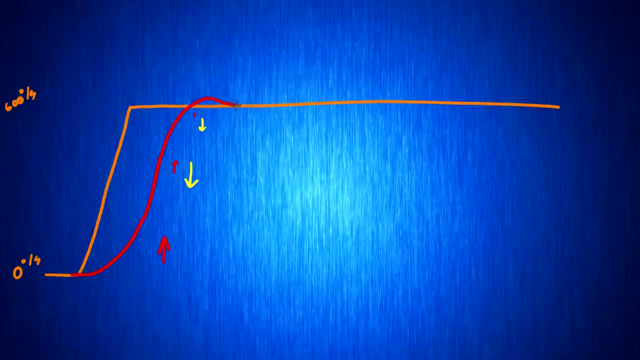 it'll really control our overshoot. And when we're on the opposite side, we've over, only overshot a little bit, and D term again starts to compensate and say, Hey, we're approaching pretty slowly, We can start slowing down. 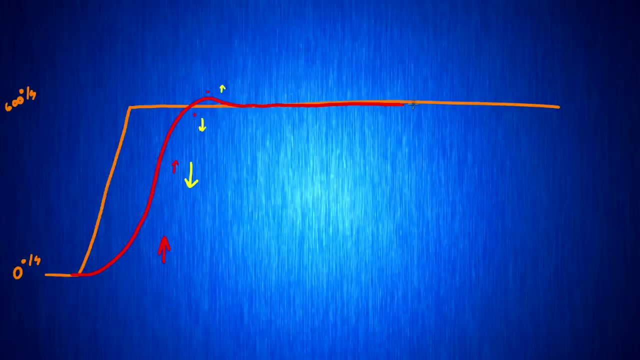 And it really damps out that overshoot. So you hit your target. If you have your D term term tuned well, it can stop um slow you down enough so that you actually hit your target without a lot of overshoots. Now, something that you'll hear a lot is how D term reinforces noise. 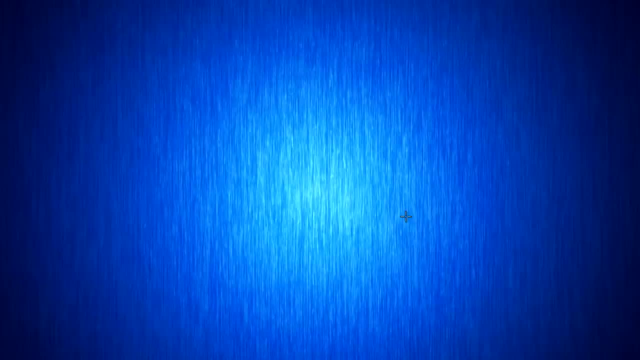 We need D term to slow us down So we don't overshoot our target, and to to to slow down oscillations, so that, rather than having a large oscillation, the D term can slow it down and maybe it'll only bounce once or twice very, uh, very small amount before it stabilizes. 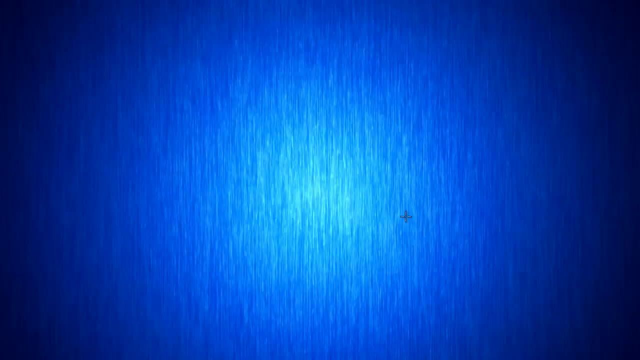 on a rapid change, Um, but if you imagine, say, we're looking at a gyro trace and we're basically sitting still and we have a little tick of noise that just goes away and comes back, If we imagine the P term, all all the while looking at this thing saying, yeah, we're dead on, we don't need. 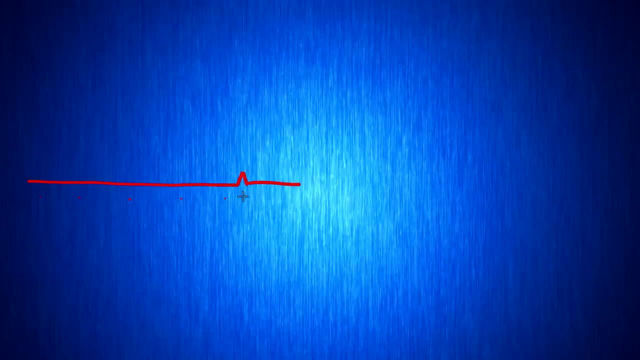 to do anything. We're dead on, We don't need to do anything. all through here We get a little bit of noise. The D term says Oh well, or P term says Oh well, we're a little bit off, We didn't. 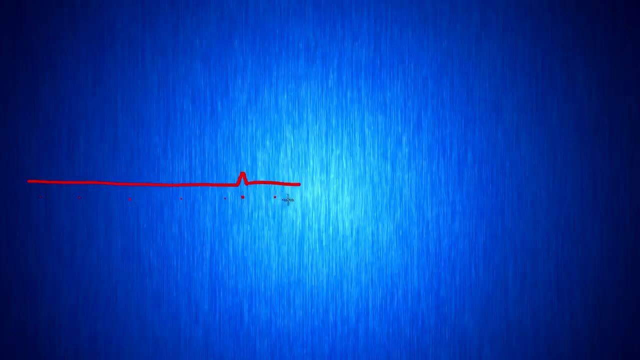 need to move a little bit there And then, Oh, we need to do nothing. So it really doesn't care about just a little um blip in the uh trace. But if we consider what the, the D term sees, 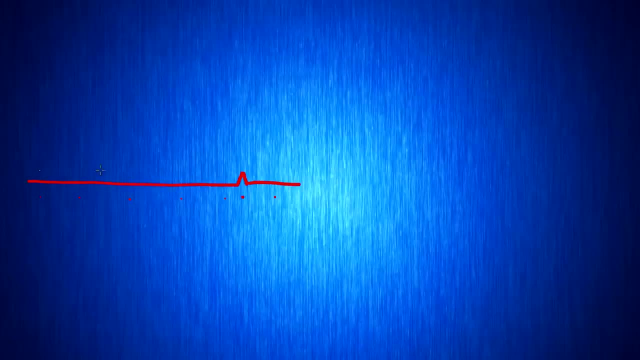 it also sees: well, we're there, We don't need to do anything, and the same at each of these locations. But when we get our blip of noise all of a sudden, it says we are rapidly moving away from our target. So the D term says: Hey, we're getting away really quick, We need to start moving. 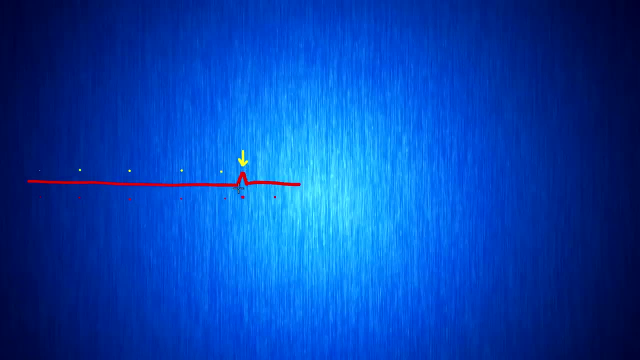 the opposite direction, to, to, to slow down this, uh, this movement away from our target, And then on the next bit, there it'll do nothing, but there'll be some delay. This doesn't happen instantly, And so this little bit of noise then becomes a motor command that later down the line, 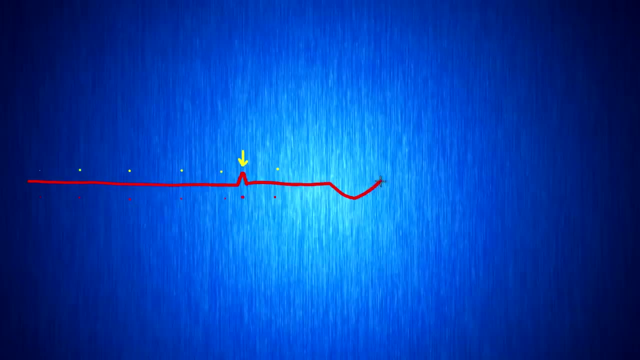 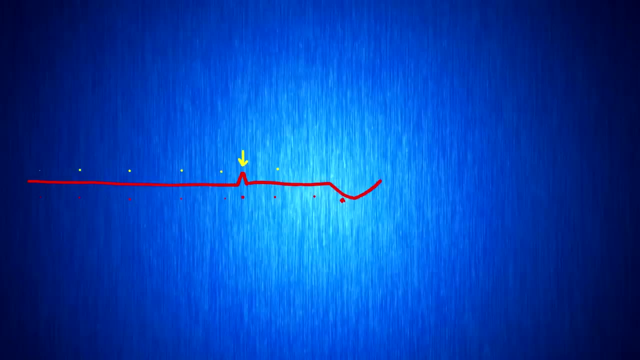 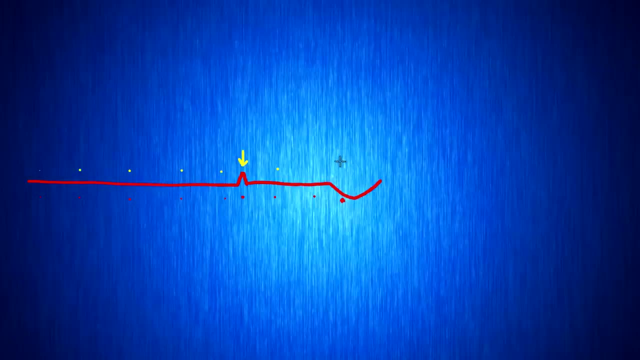 moving away from our target really quickly. We need to start moving this way. We need to start moving this way. And again, we've got a bit of a delay before these motor commands start coming down and we can get where one little blip of noise can cause the D term to get overexcited. 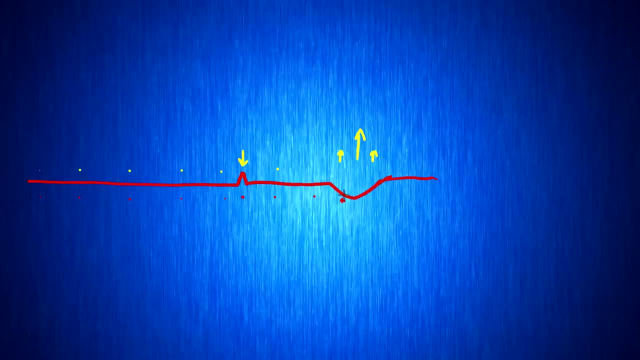 and cause large motor movement. That then cause other motion and, uh, ends up giving a really jittery. You see, the, the where your motors are jumping around and the D term is, is up and down all the time, So that's why it's. 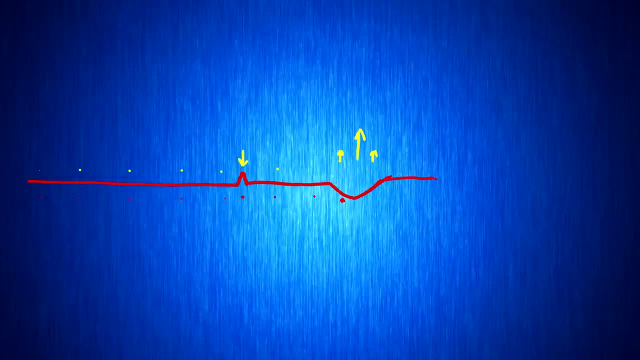 really important to to control noise, because a little bit of noise in your gyro trace, say you've got an unbalanced prop or something like that. The D term is going to see all of these, as you know, differences in speed. It's we're going to be accelerating and 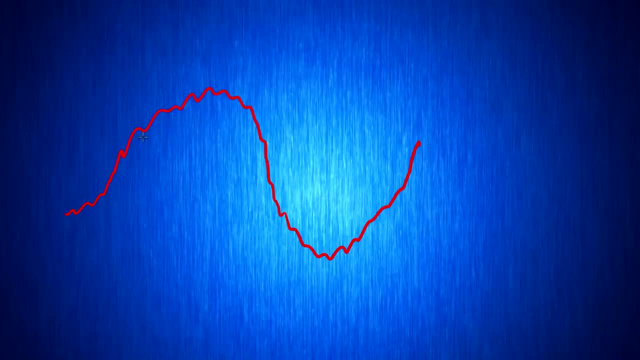 and breaking towards our our target this whole time And it's going to really overreact to that. So that's where filtering helps a lot. Um and uh, try and doing physical things to mitigate noise. uh, doing soft pads on the motor, soft mounting your FC um O rings are really commonly used. 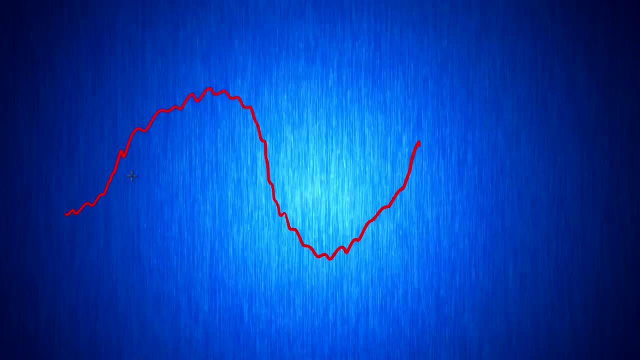 that sort of thing because we need to use the D term to compensate for the P term. So if we turn, if we have a lot of noise and we turn the D term down, then the P term is a lot more free to oscillate and overshoot And we can't use as strong of a P. 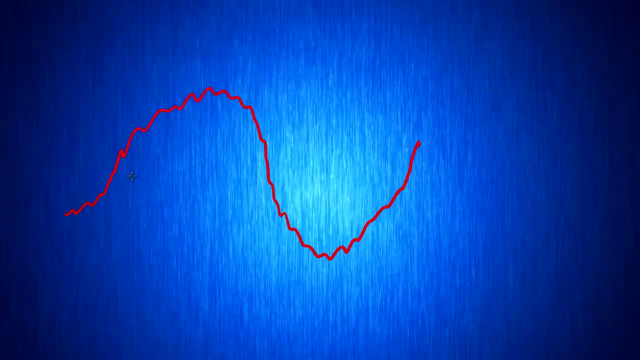 term because we don't have the D term. reigning it back in The final term is the I term. The I term happens over a long period of time And what happens is, if you have your, your P term, say you're, you're very close to your target. the P term is just a tiny, tiny amount of strength. 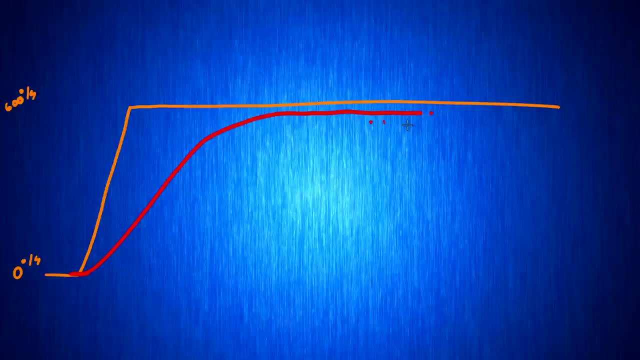 And it's not necessarily enough to push us to exactly, to actually hit our target. So what the I term does is it looks over this long period of time and says, Hey, we're not actually quite at the destination yet, And it helps apply an additional 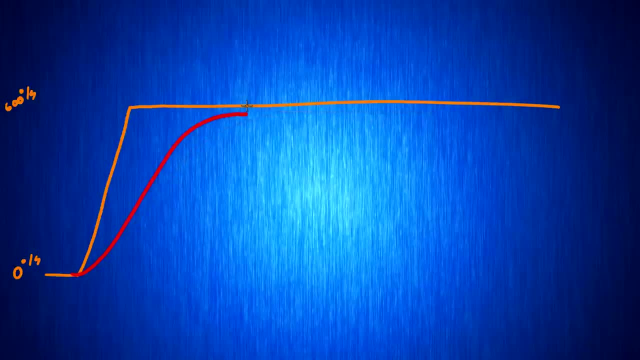 force. So if we are hitting near our target, our P term is saying, yeah, we're basically there, We don't really need to move, And the I term can say, no, we're not quite there yet, We need to. 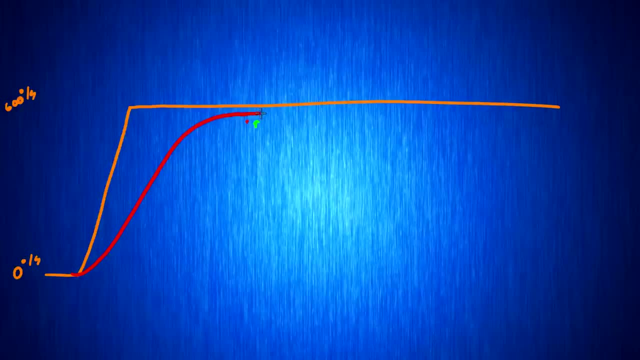 start pushing up, but the I term is very weak. So if we're hitting near our target we're not weak, So it only pushes us a little bit. And then when we check again, we're still getting basically nothing out of our P term. but the I term says no, we're still not there yet. We need to go a.